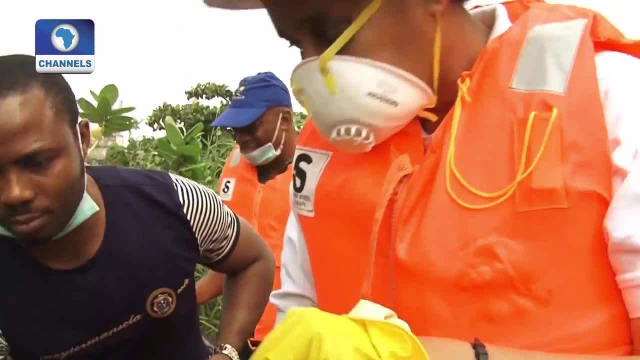 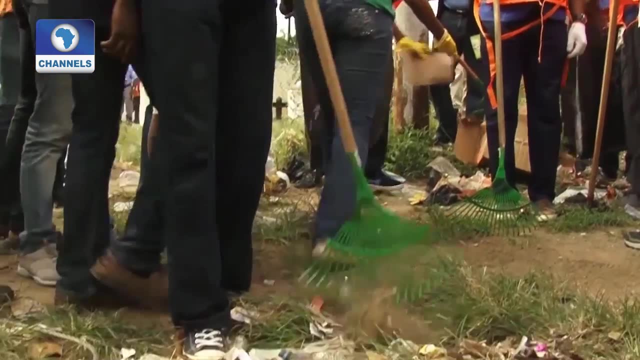 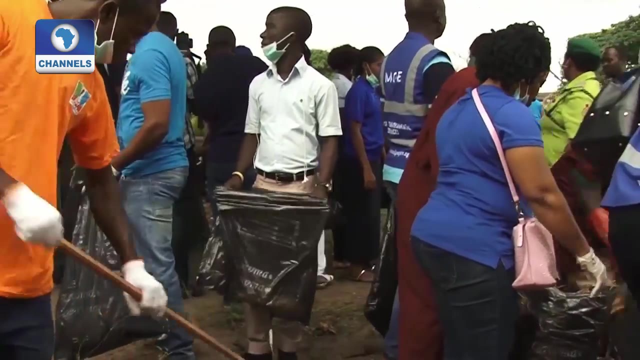 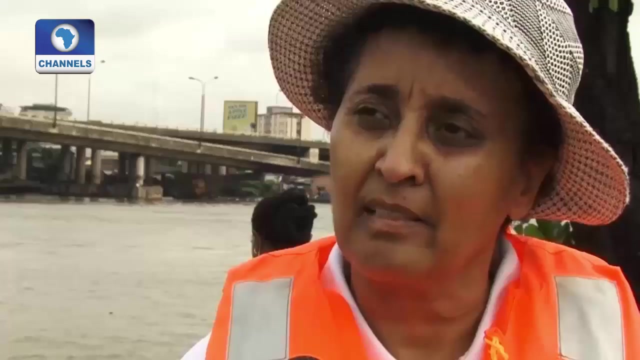 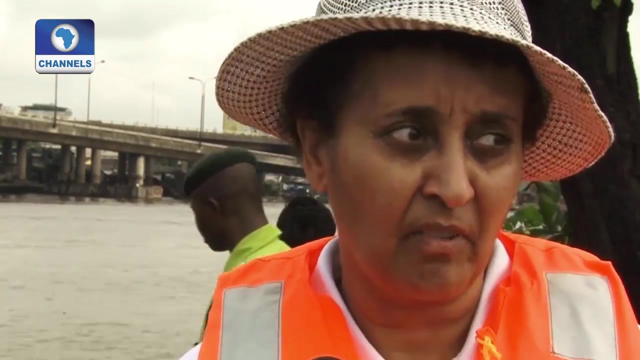 Environment, Lagos State and other volunteers together cleaned the shore. What we're doing today, you know people are getting together in the United States, in China, in other places just doing this, And the purpose is not only to clean up this environment, the immediate environment, that 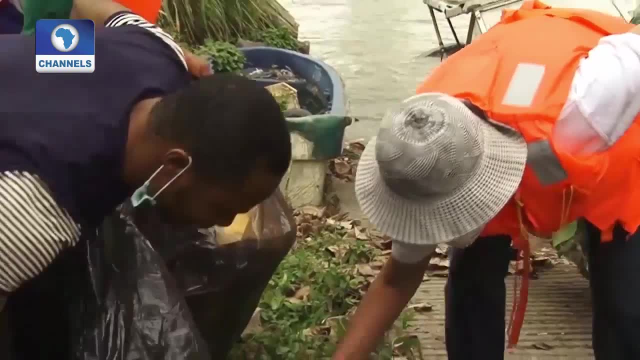 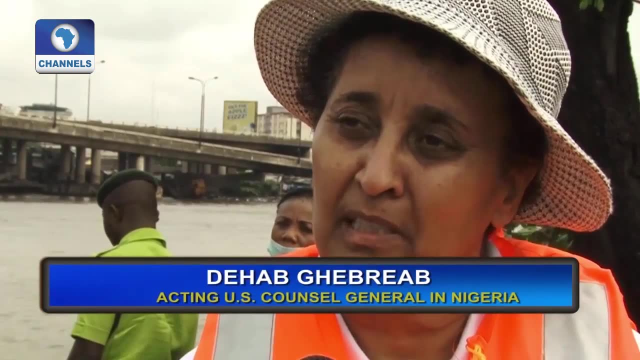 we see here. but beyond that, the increased awareness that the plastics that we drop as we move forward doing our daily business affects the environment that we live in, So it's really critical to, in order to have a sustainable planet, we need to take care. 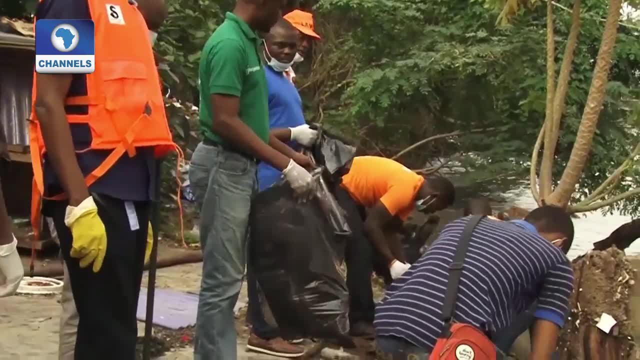 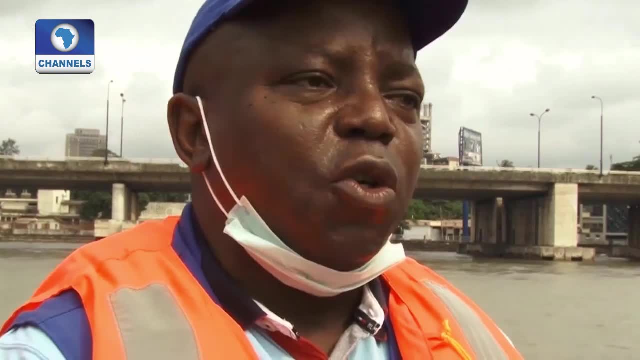 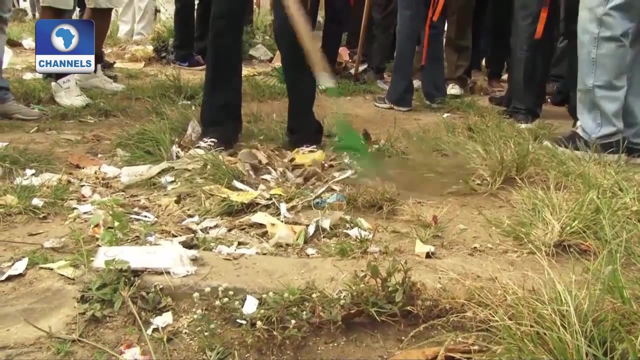 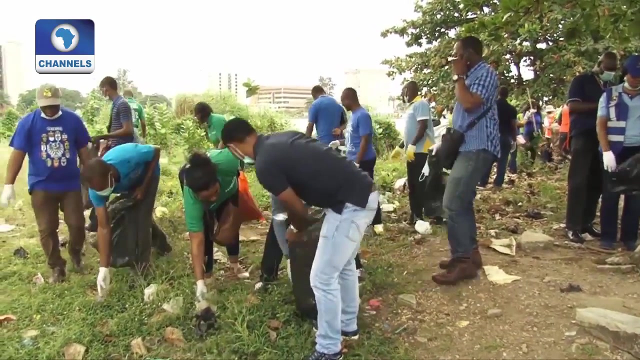 of it And ensure that they don't drop their waste inside our waterways. We want them to ensure that the plastic bottles that they use don't end up in our waterways. They are harmful to our water. Sorry, I want to do that. 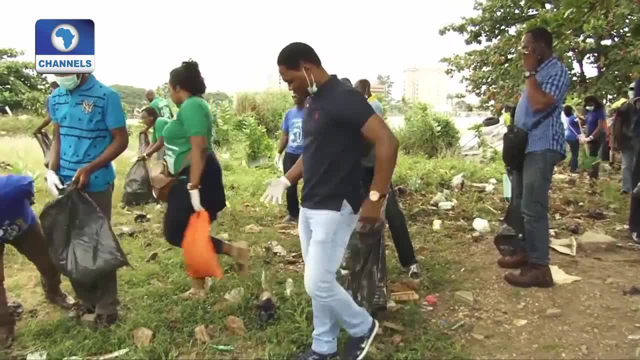 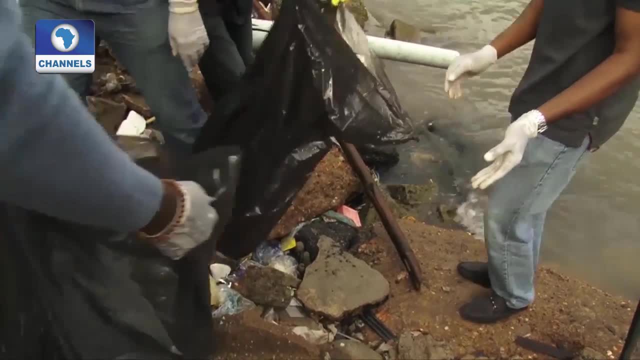 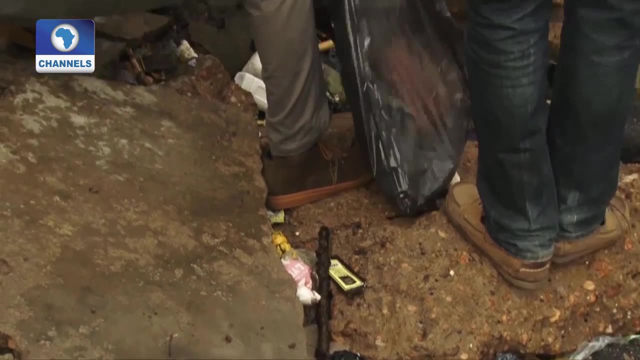 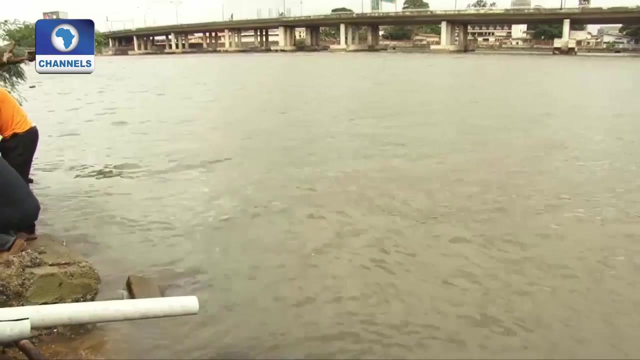 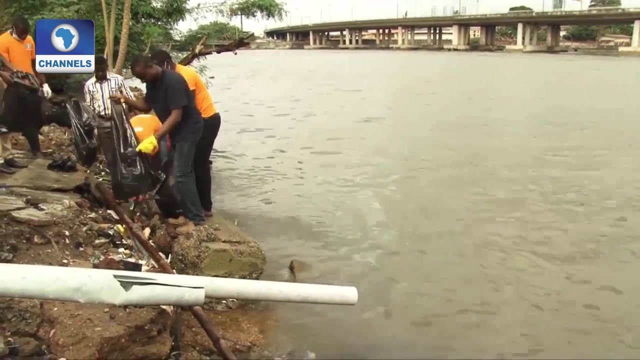 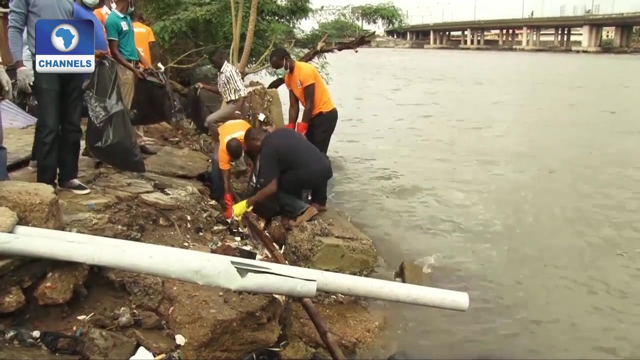 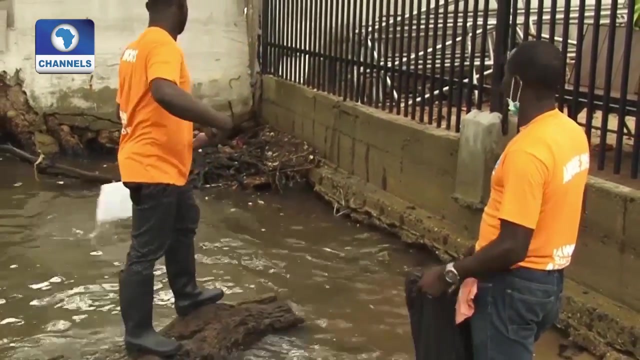 Hold that up, please Hold that up. please Hold that up, please. You want? Okay, okay, It's time to go. Okay. Some volunteers appeal to the people to refrain from dumping any type of waste into the ocean. 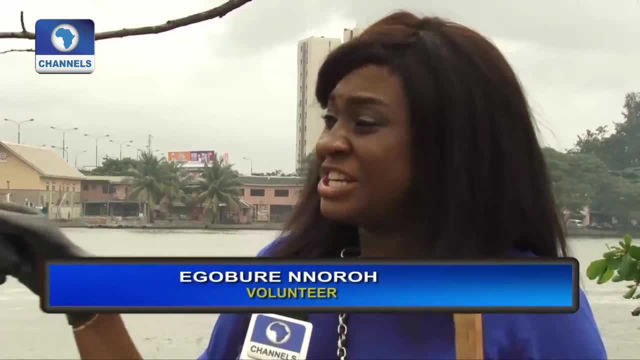 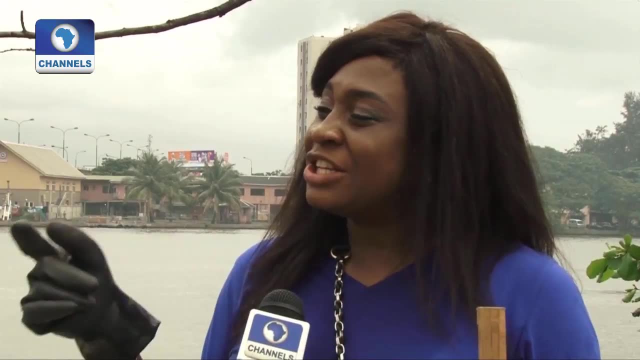 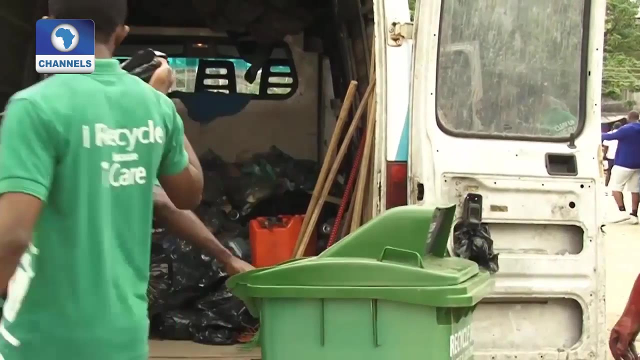 There are inhabitants in this water. You don't need to pollute the environment. one Two: they shouldn't defecate or urinate along these coastal areas. At the end of the event, all participants agree that proper disposal of waste will improve the health of the people, wildlife and the local economy.